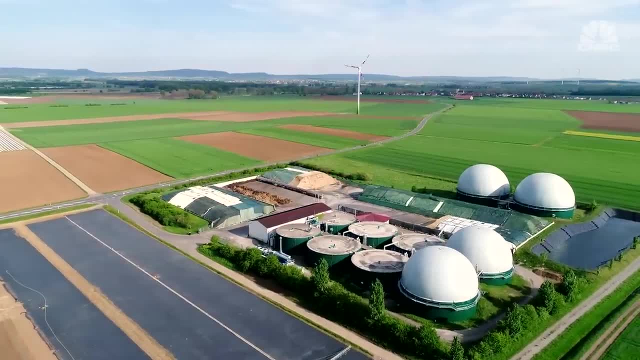 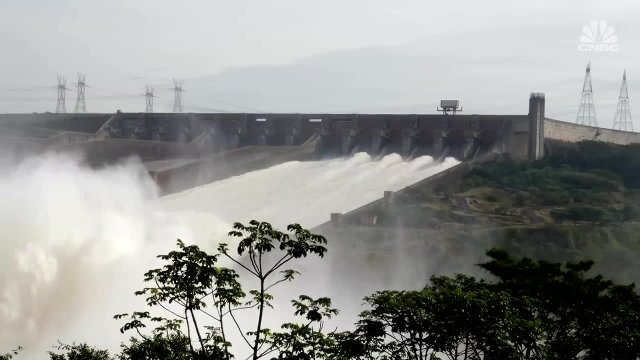 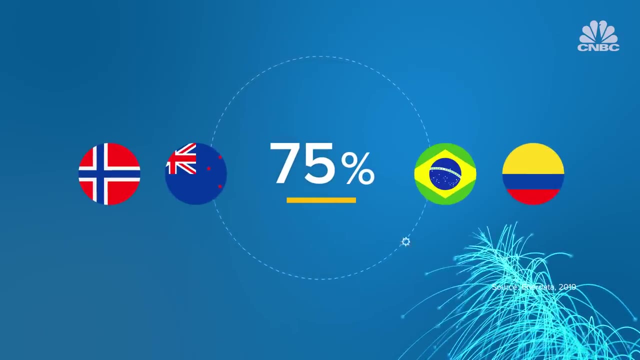 But the most telling metric is likely the role of renewables in a country's overall energy mix. Nordic and Latin American countries have a good showing on this list. More than 75% of Norway, New Zealand, Brazil and Colombia's energy production comes from renewables. Venezuela. 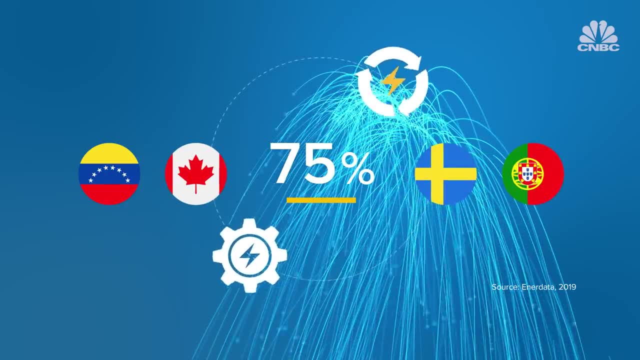 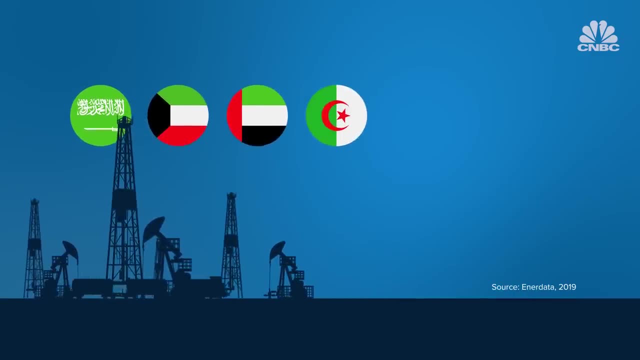 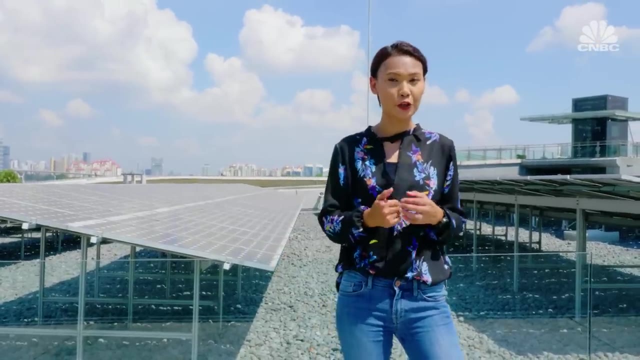 Canada, Sweden and Portugal also make a good showing, But for big oil-producing nations like Saudi Arabia, Kuwait, the UAE and Algeria, renewables are unsurprisingly near non-existent. But again, not all countries have equal geographies and policies. Think of renewable energy as 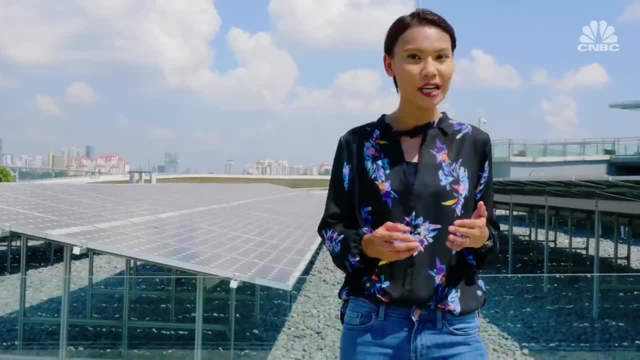 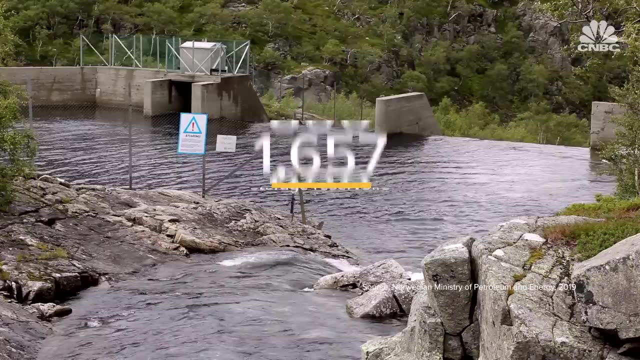 something bespoke, with each country harnessing the environment according to its unique surroundings. Norway has 1,660 hydropower plants and more than 1,000 storage reservoirs. It is possible for Norway to depend on hydropower because of the country's 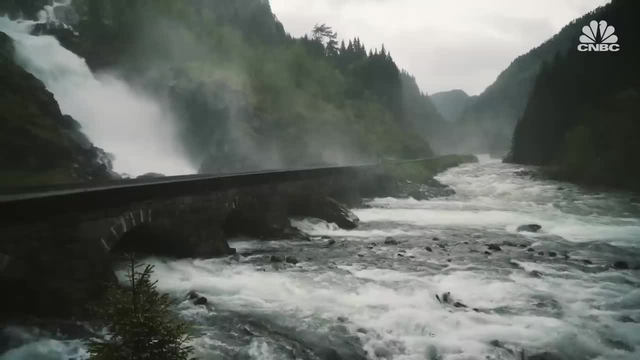 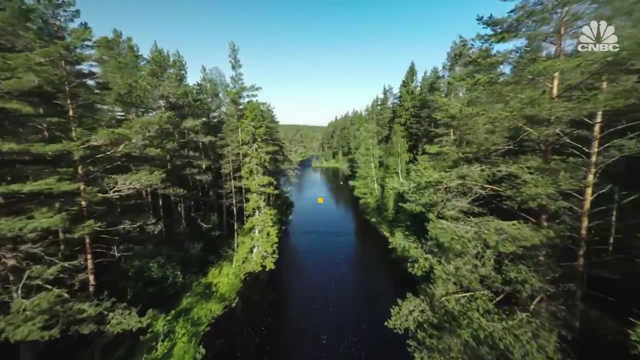 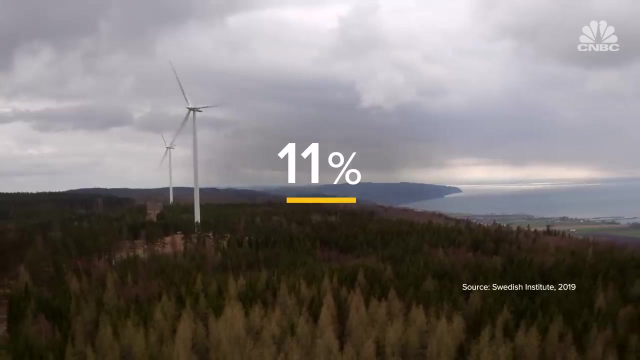 long coastlines, steep valleys and high levels of running water. In neighbouring Sweden, where forests make up 63% of its land, mass bioenergy is increasingly being used for heating as well as for electricity production: 11% of its electricity is also derived from around 3,600 wind turbines. 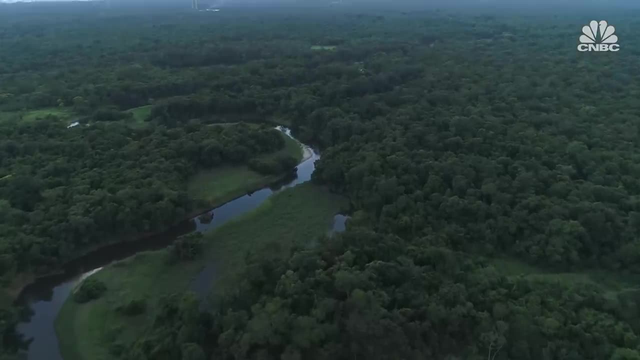 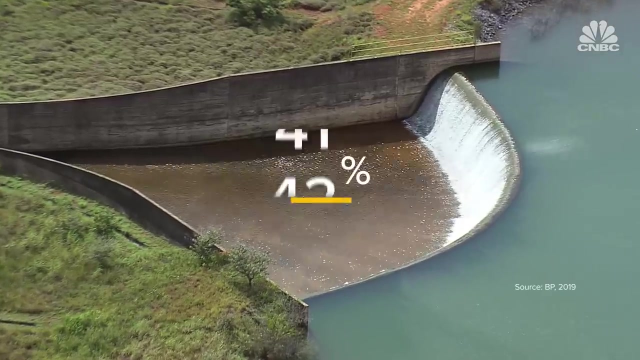 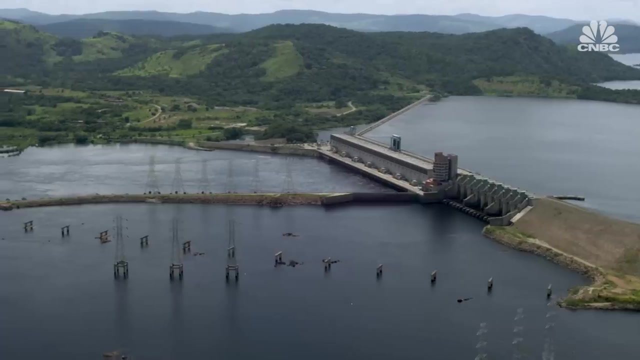 Likewise in Brazil, which has rivers and huge swathes of the Amazon rainforest within its borders. clean energy, including hydropower, accounted for 42% of its electricity production in 2017.. Ditto for Colombia and Venezuela, countries known for hydroelectricity. 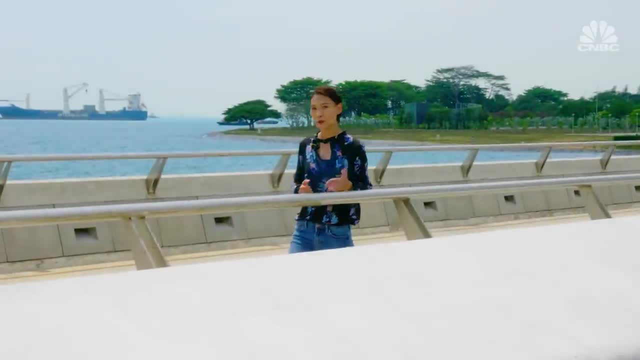 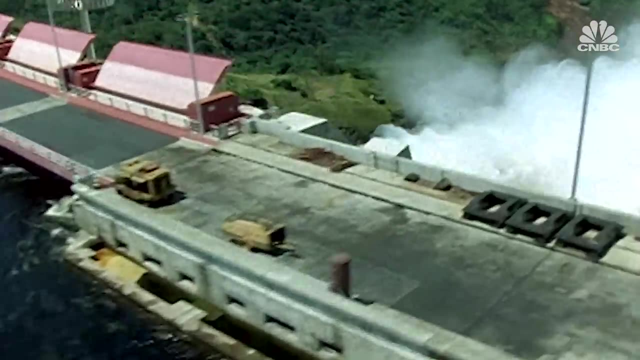 One of the famous cautionary tales about over-reliance on one form of renewable energy comes from Venezuela, which depends heavily on the Guri Dam for about 60% of the country's electrical needs. In 2010 and 2016, droughts caused the dam's water to drop. 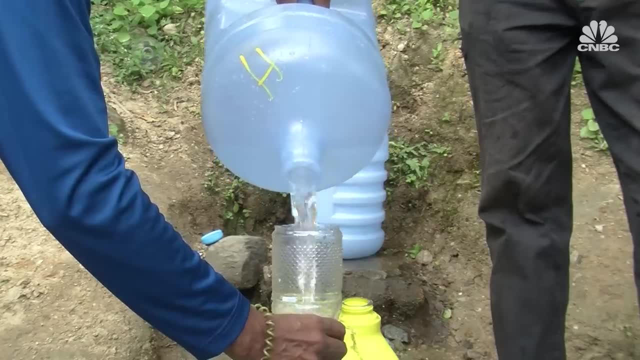 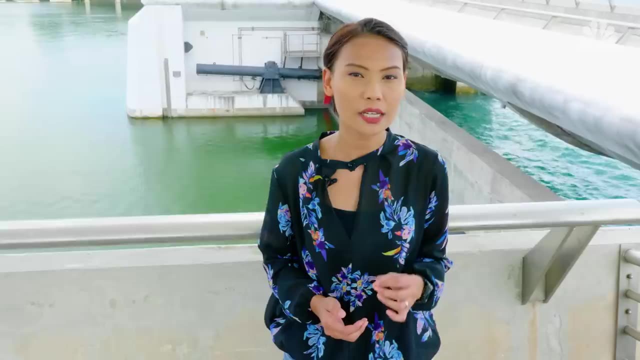 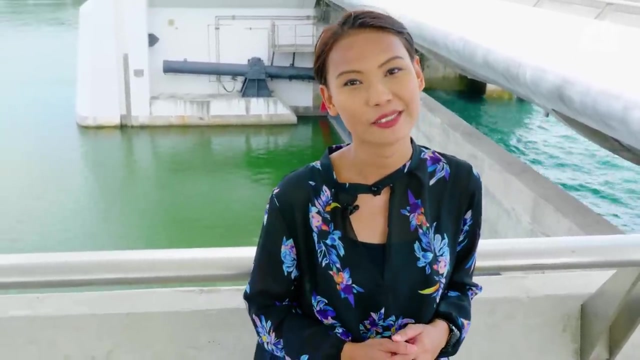 The dam's water to fall so low, the government had to declare emergencies. So where does the energy race go from here? Well, an increasing number of countries are recognising the urgent need to tackle or slow down climate change. Investing in renewable energy is one of the major steps. 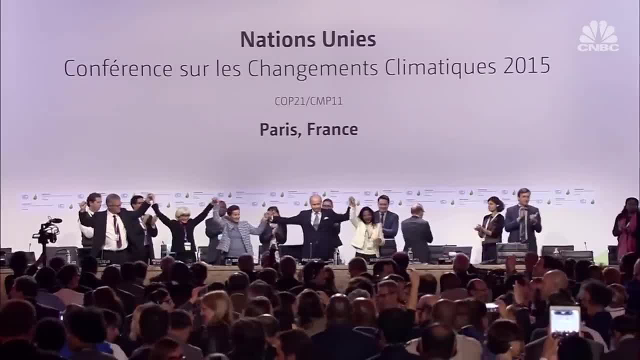 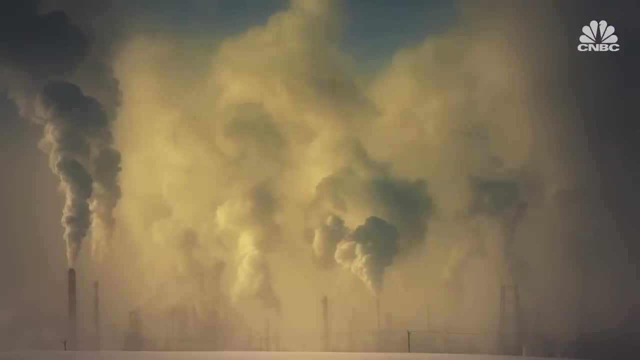 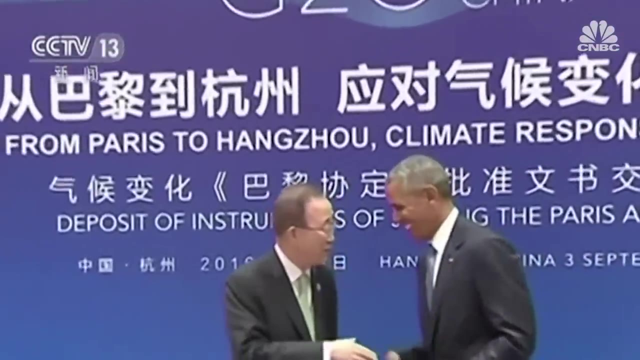 From the Kyoto Protocol to the Paris Agreement. an increasing number of signatories are joining international environmental agreements to lower emissions of greenhouse gases. The Paris Agreement brought together 195 nations to tackle climate change in 2015,, so it has had a few setbacks since. 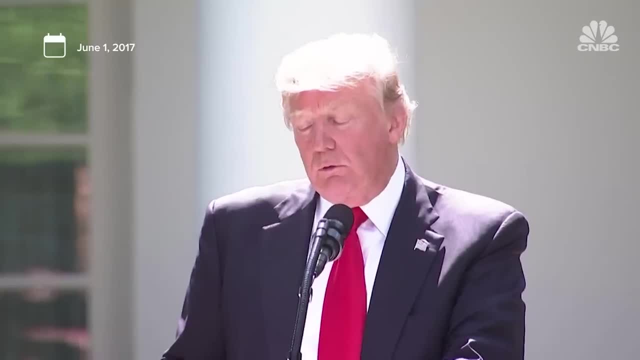 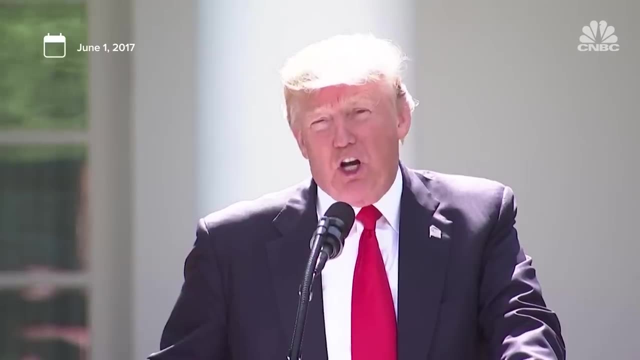 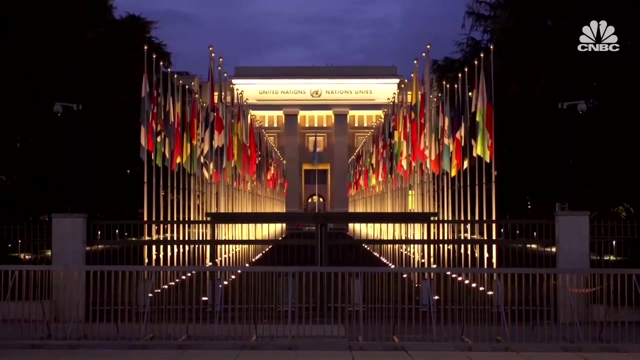 The United States will withdraw from the Paris Climate Accord. so we're getting out, But we will start to negotiate and we will see if we can make a deal that's fair. Other targets include the UN Sustainable Development Goal for affordable and clean energy. 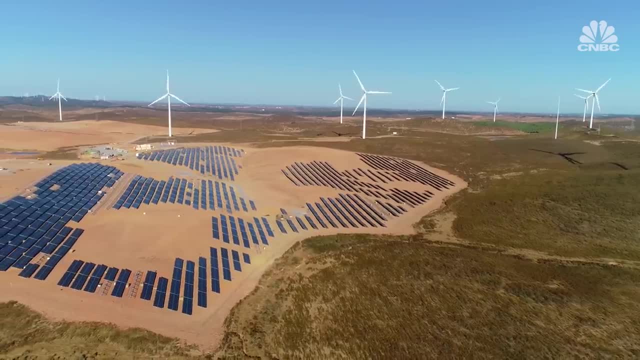 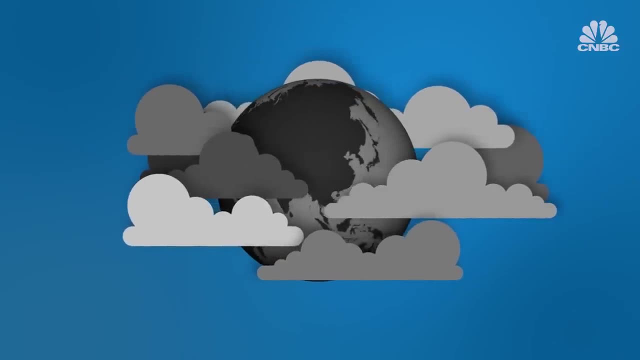 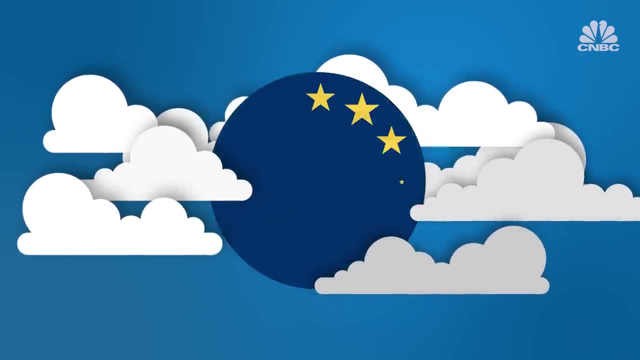 which includes increasing the share of renewable energy in the global energy mix by 2030.. In the meantime, countries have set unilateral targets as well. More than 60 countries are planning to bring their carbon footprint to zero by 2050,, with the European Union aiming to become. 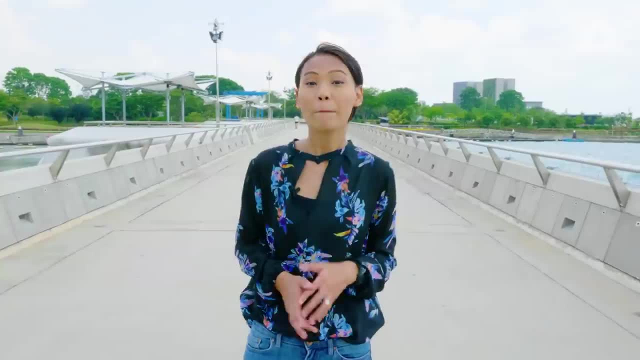 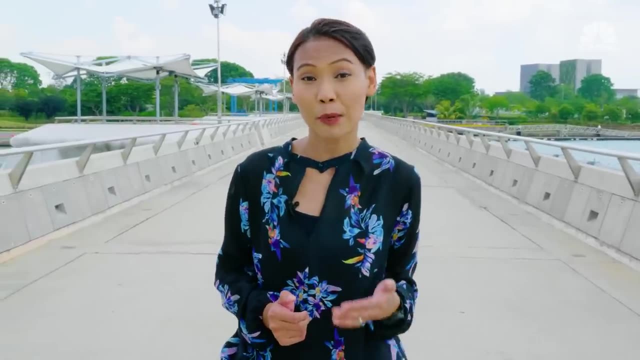 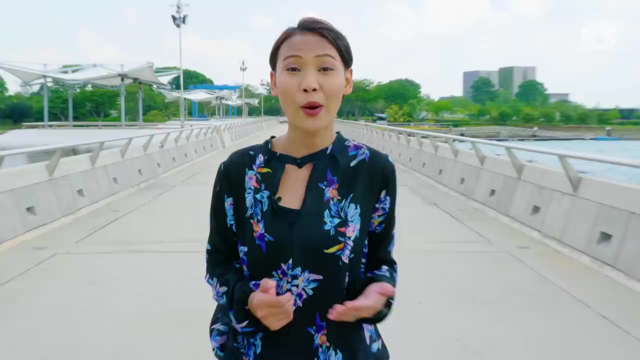 the first climate-neutral economy, But most renewable energy sources are still subject to unpredictable forces of nature. Imagine a drought rendering a dam useless and taking out a country's sole electricity supply, or intermittent energy from wind or solar sources. What then? That's where innovation and new technologies kick in. 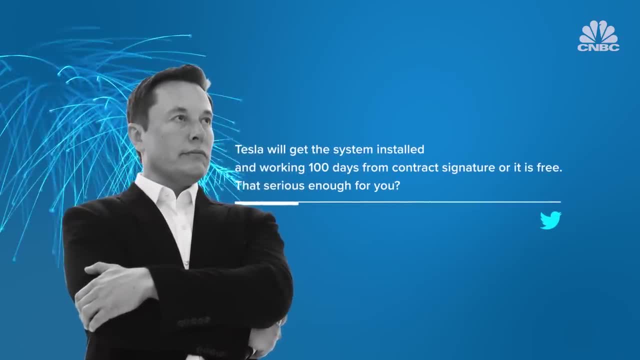 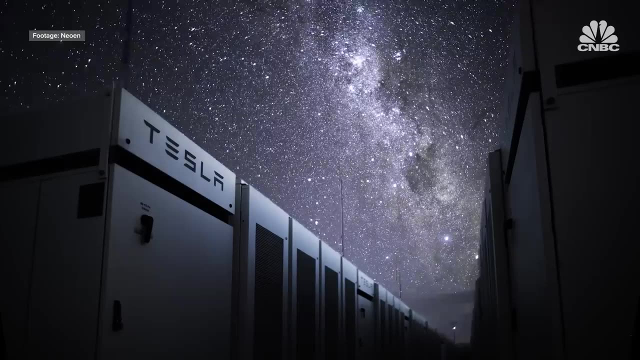 Remember when billionaire Elon Musk tweeted that he would install a battery storage system in South Australia within 100 days or deliver it for free? The Tesla battery system now holds the title for the largest lithium-ion battery in the world. It's the largest lithium-ion battery in the world. 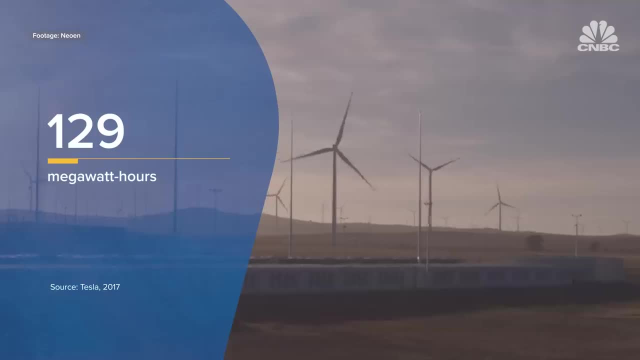 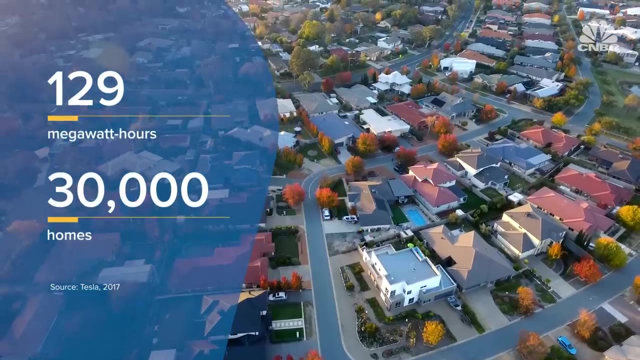 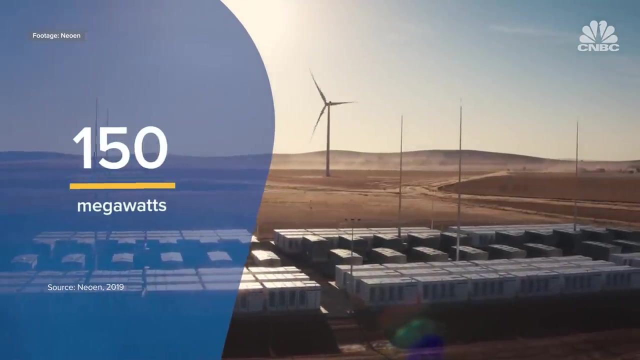 It can currently store 129 megawatt-hours of energy from wind turbines by renewable power company Neowen. This is enough to meet the needs of 30,000 homes. Now, Neowen has plans to upgrade its capacity by 50% to 150 megawatts. 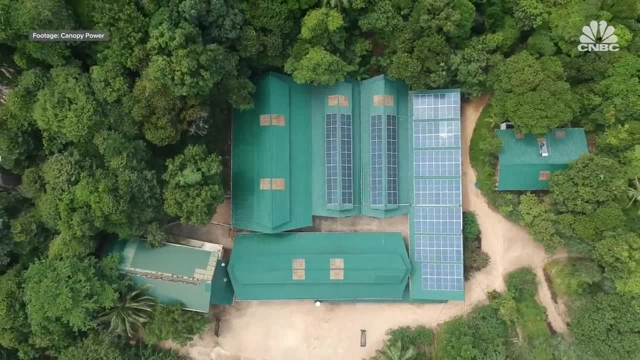 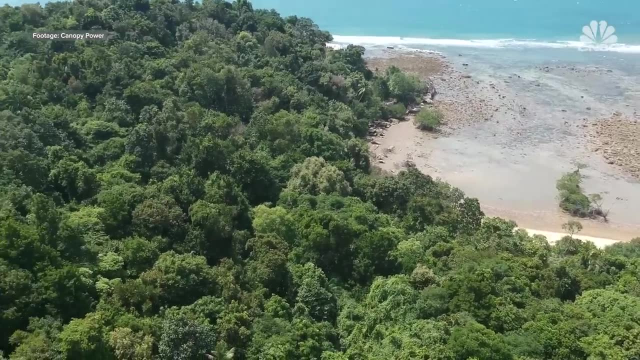 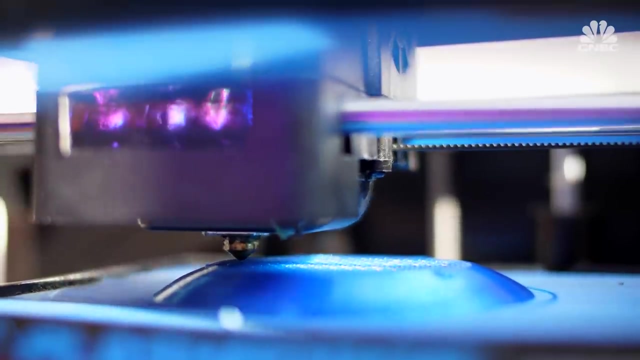 More localised microgrid systems are already powering remote locations like these far-flung islands in Southeast Asia and providing reliable energy storage. To power the world with renewable energy. we're going to need much more storage than that. 3D printing is seen as a way to reduce the cost.